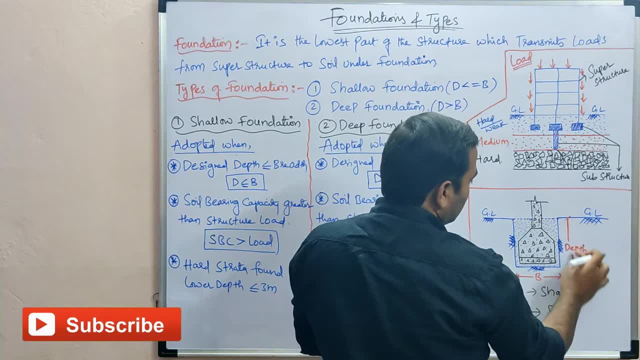 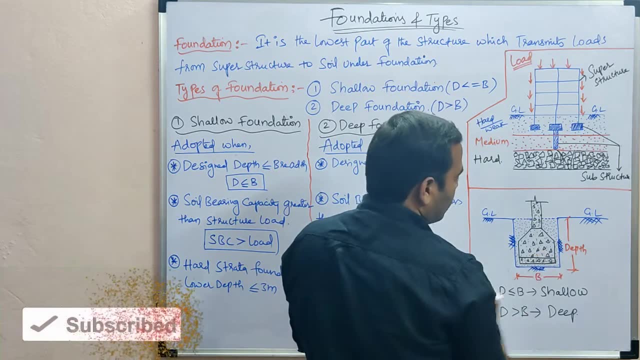 have taken this ground level and I have taken this ground level and I have taken one footing and this is the depth of foundation. so depth of foundation is nothing but from top of surface to bottom of this excavation, that is bottom of footing. this is depth of foundation and this is breadth of foundation. that 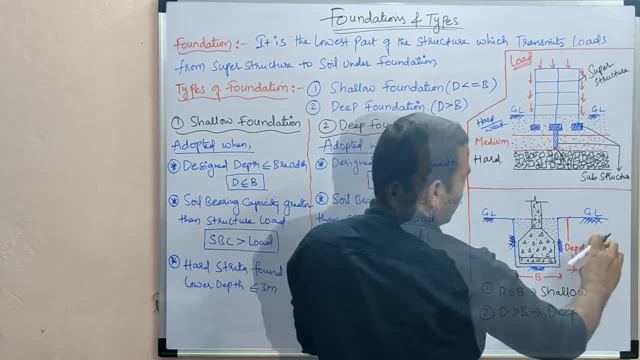 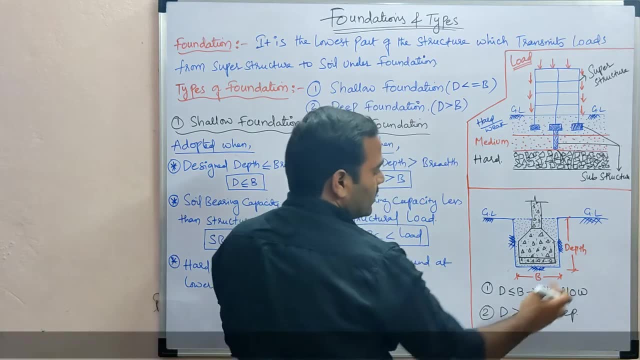 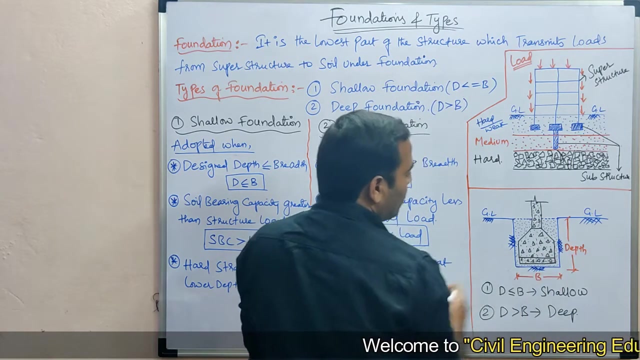 is nothing but the breadth required for this footing. if depth is less than or equal to bread, then we call it as a shallow foundation. next one is: if this depth is greater than the breadth, then we call it as a deep foundation. so, based on this dimension and based on the design, so we 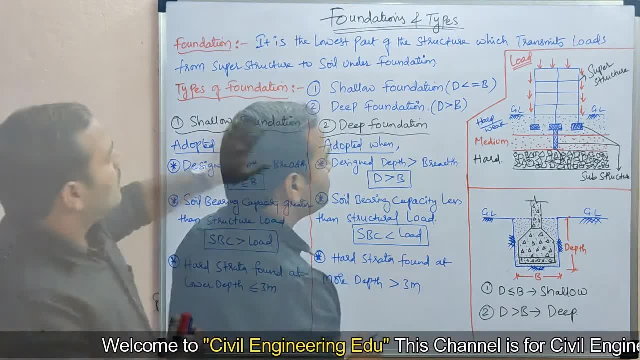 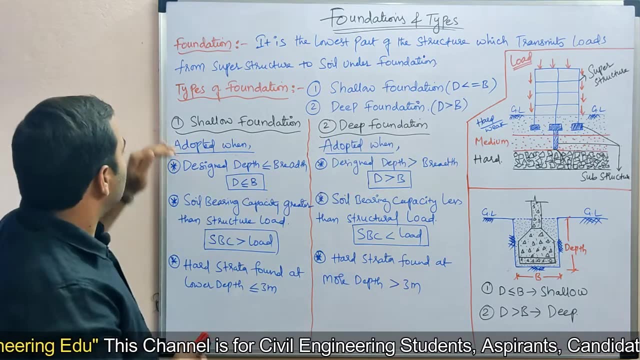 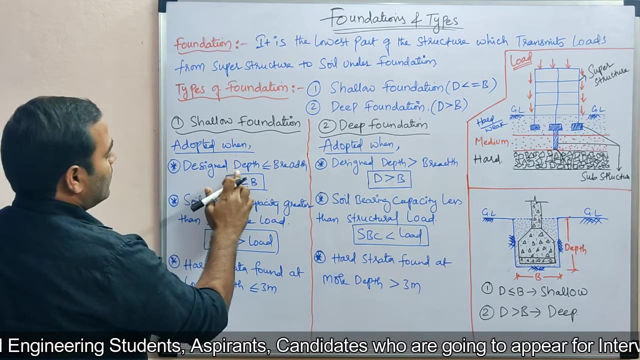 are going to divide this into two types. types of foundations are shallow foundation and deep foundation, based on this condition and soil bearing capacity, so shallow foundations are adopted when these three conditions are seen here. so design depth is less than or equal to breadth, then we are going to opt shallow. 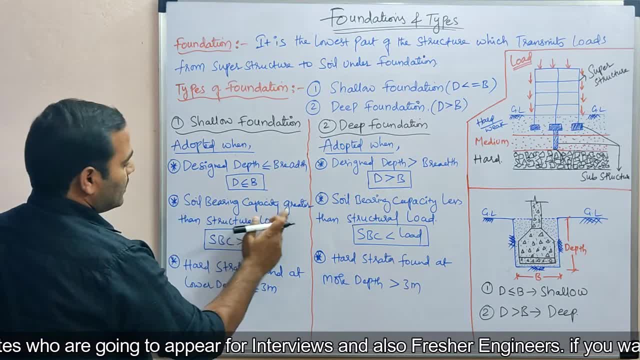 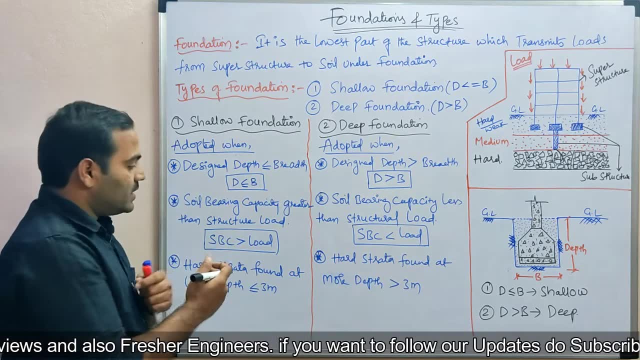 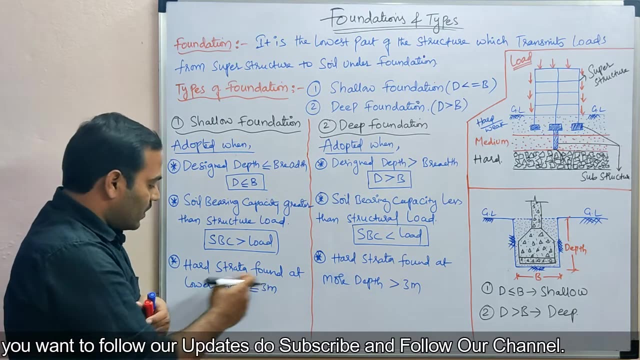 foundation. next one is soil bearing capacity is greater than the structure load. so when the soil bearing capacity is more and the structural load which is acting is less, so then we are going to follow this shallow foundation next. third condition is hard strata is found at lower depth, that is. 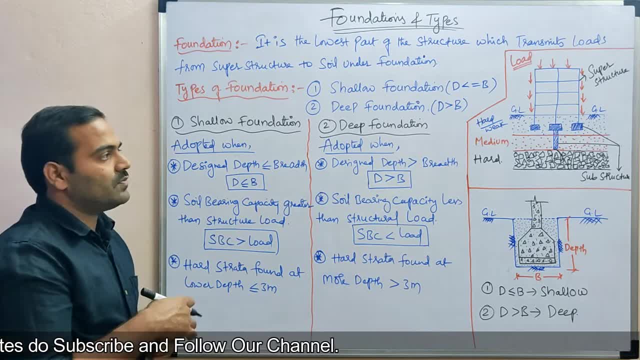 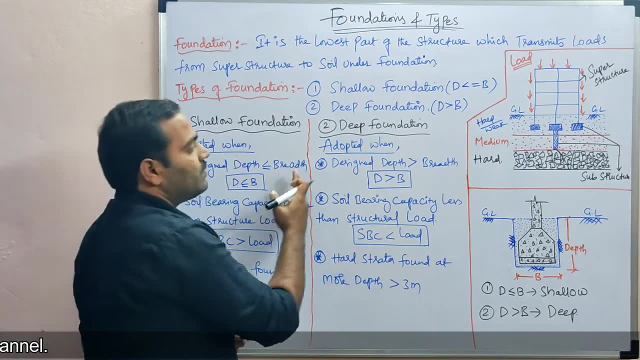 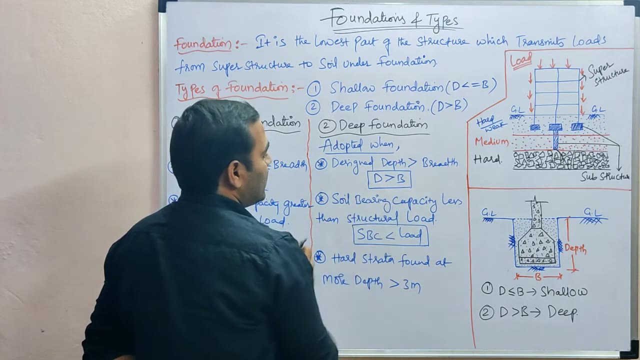 less than or equal to three meters. if the hard strata is found at lower depths, then we are going to opt to this kind of shallow foundation. next one is deep foundation. this kind of foundation is adopted when designed depth is greater than the breadth. this is the first condition, and second one is soil bearing capacity is less than the structural. 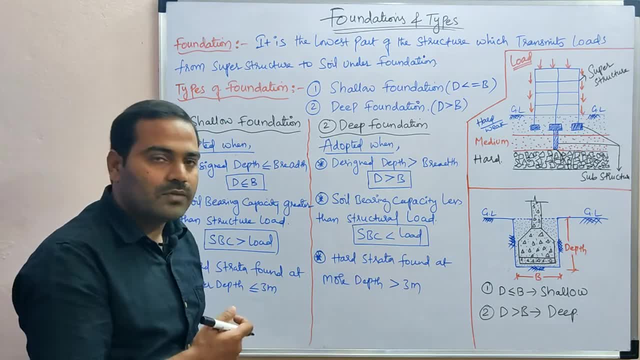 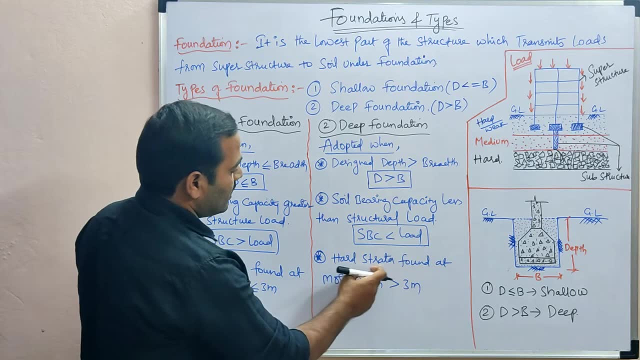 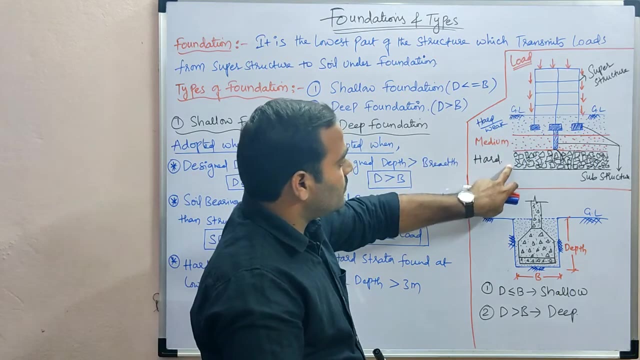 load. that means sbc is less when compared to that of structural load. in this case also, we are going to opt deep foundation. next third point is hard strata found at more depth. that is, greater than three meters, if you see here. hard strata is found here, so that is the. 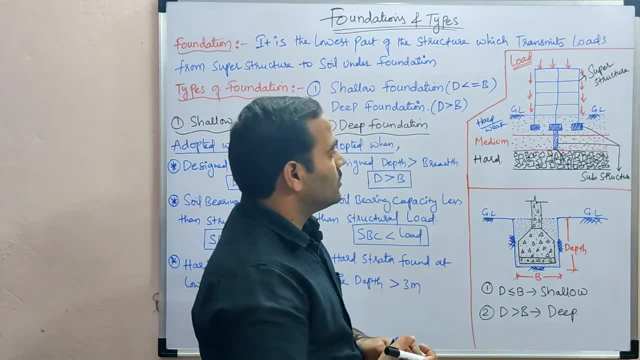 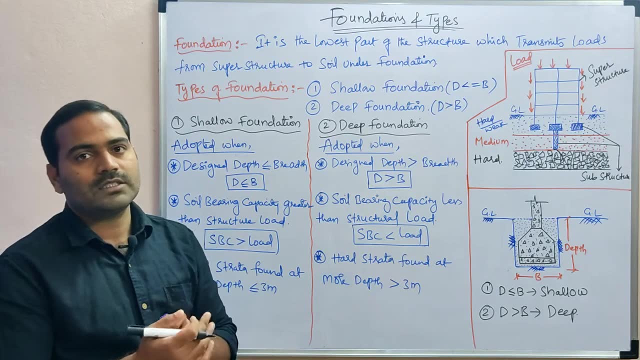 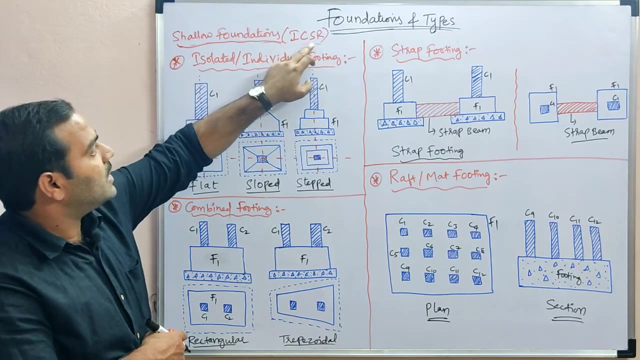 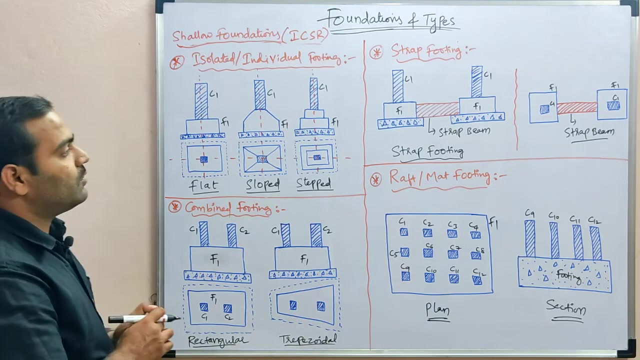 reason we have taken this type of foundation. so this is that point. so, based on these conditions, we are going to differentiate what is shallow foundation and what is deep foundation. so these are the different types of shallow foundations. so shallow foundations can be remembered like this: icsr, isolated, combined strap and raft, or mat footing. so these are four different. 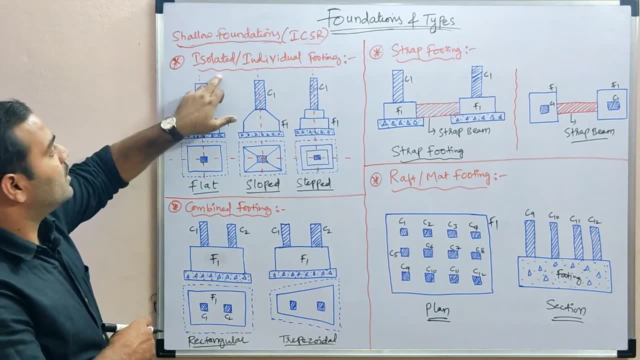 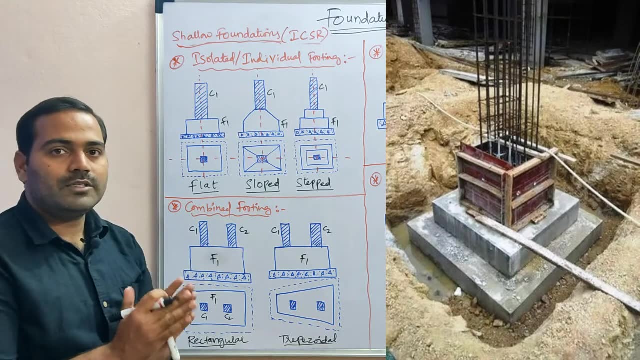 types of footings. so if you take first one, it is a isolated footing. it is also called as individual footing. so in the heading itself we can understand that it is individual type of footing. that means under every column there will be a separate footing. so isolated footings. 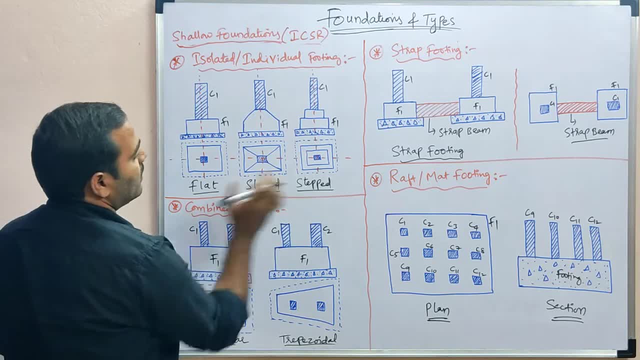 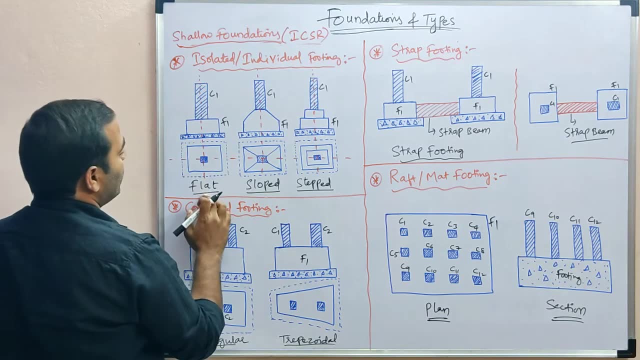 are again divided into three different types. this is first one, second one and third one. so if you take first one, this is the plan shown here and this is the section. so in this flat footing- so that footing will be completely flat- there will not be any slope or step. second, 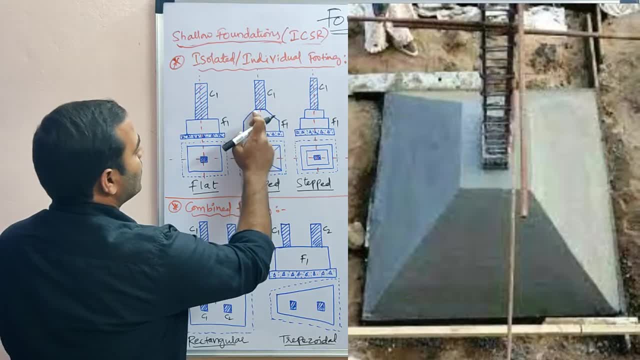 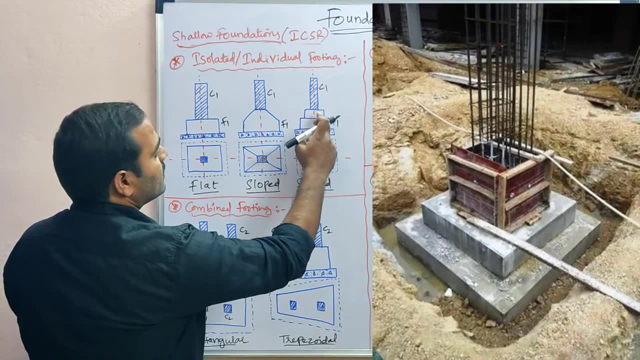 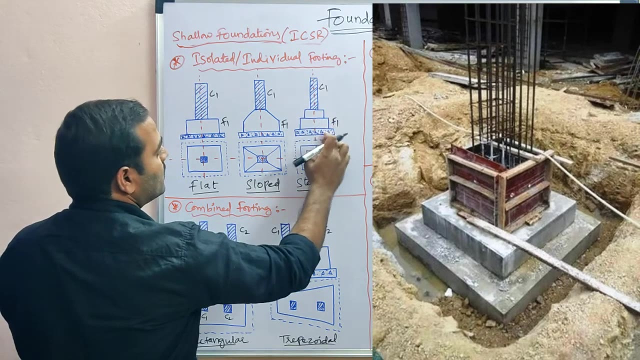 one is slope approach footing. so in this sloped footing we can see there are slopes given here. third type of footing is stepped footing. so here this is step one, step two. in some cases step three also will be there. so this is the column, these are two steps and this is pcc. footing is one, column is one. so these are. 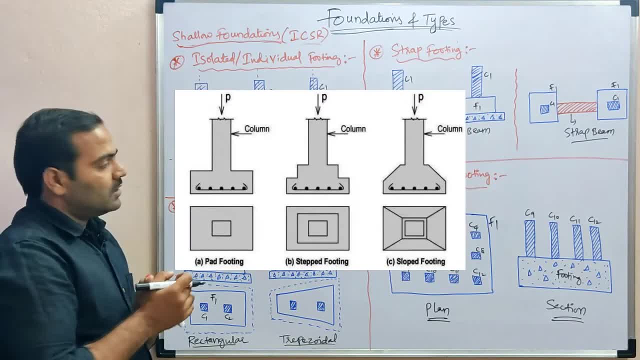 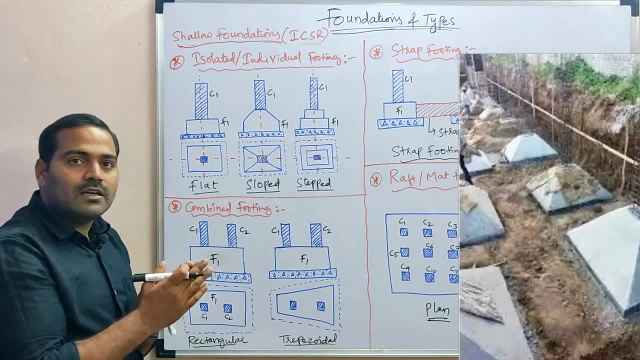 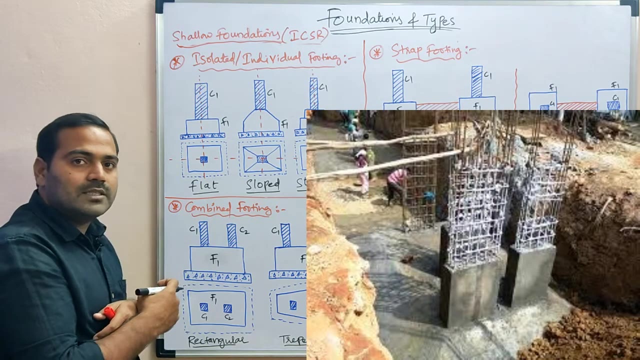 called individual or isolated type of footings. so second one is combined footing. so in isolated footings, when the distance between column footings are more, then in that cases we will lay separate footings. when the distance between two column footings are very less, in these cases we will do: 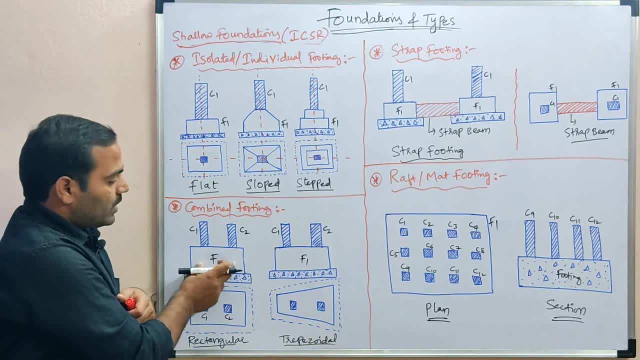 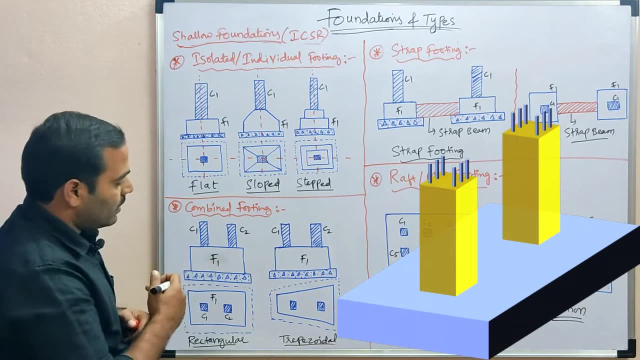 the combined type of footing. so in combined footing the footing will be one, columns will be two. that means, two columns will be laid on a single footing. so here also you can see two columns and one footing. so these type of combined footings are again divided into. 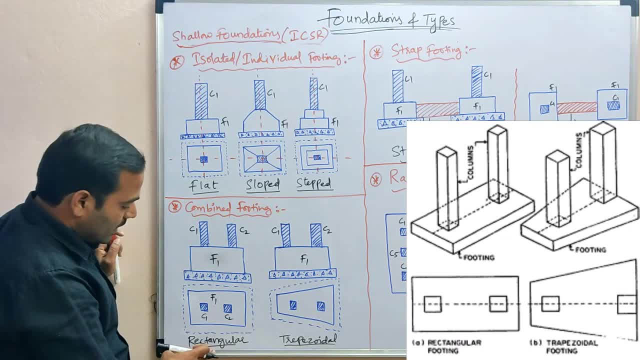 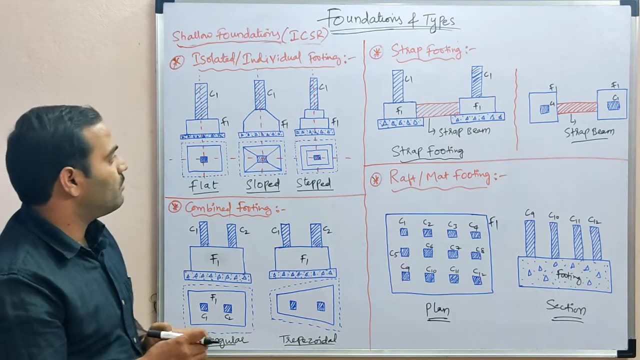 two different types based on their shape. first one is rectangular type, so the shape of the footing will be rectangular and two columns will be laid over it. second one is trapezoidal type, because the shape of the footing is trapezoidal. so these are the two different types of combined 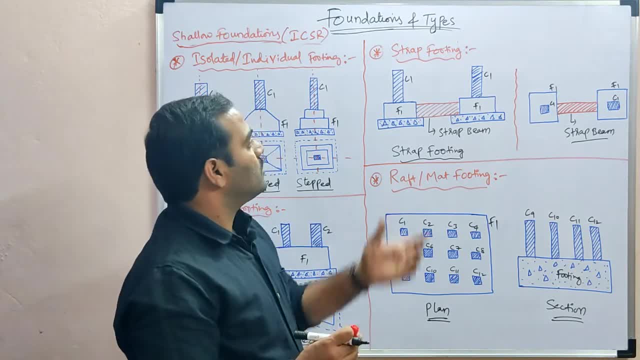 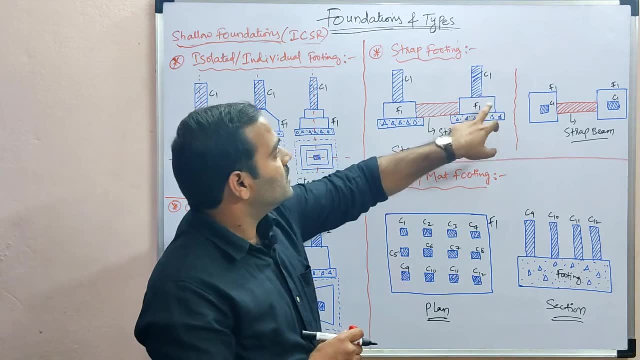 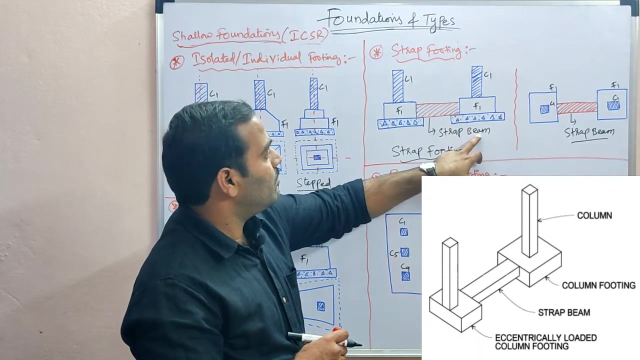 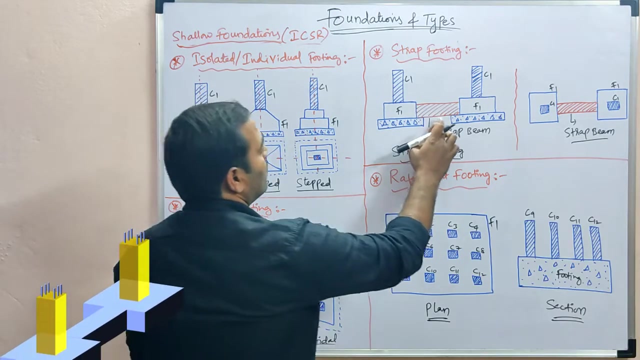 footings. now coming to strap footing, so this is also similar to that of a combined footing. but what will happen? this is single footing, this is single footing and these two single footings are connected with a beam. this beam is called as a strap beam. why this beam is connected? because to strengthen that two individual footings, a beam is connected. 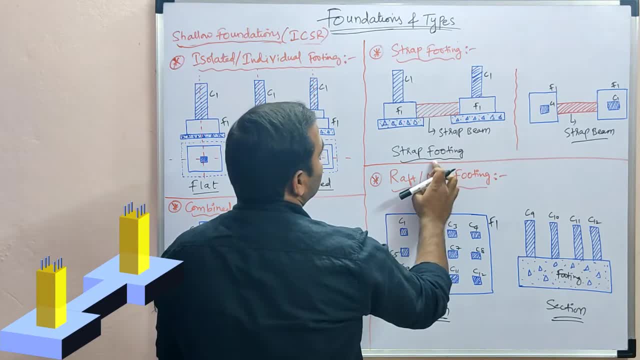 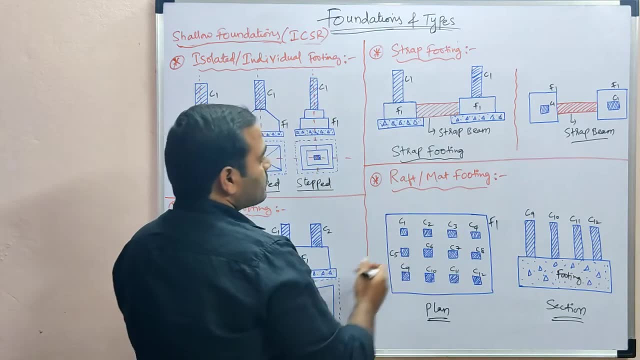 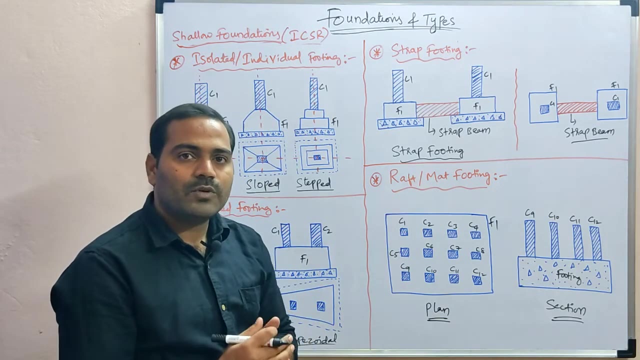 so this beam is called as a strap beam. so that is the reason this type of footing is called as a strap footing. so this is the sectional view and this is the plan view. coming to raft or mat footing, so when the soil bearing capacity is very low and area of the footing is 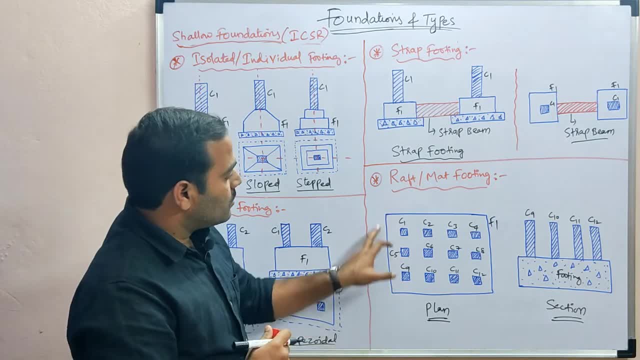 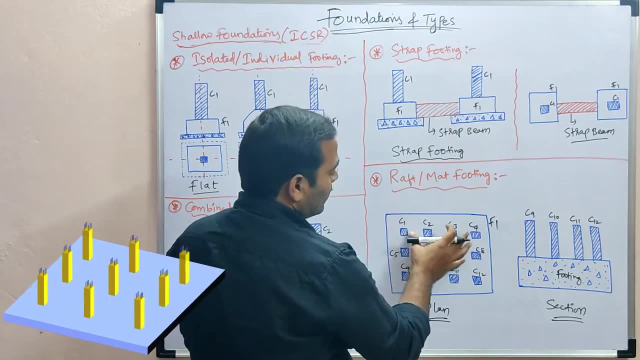 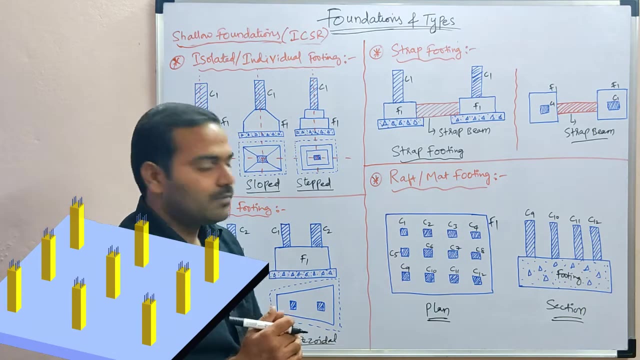 more so in such cases, what we will do. so we will lay this kind of complete footing and over this we are going to lay different columns, so all the columns will be laid on a single footing. so this footing will be laid throughout the plot area. so this type of footing, 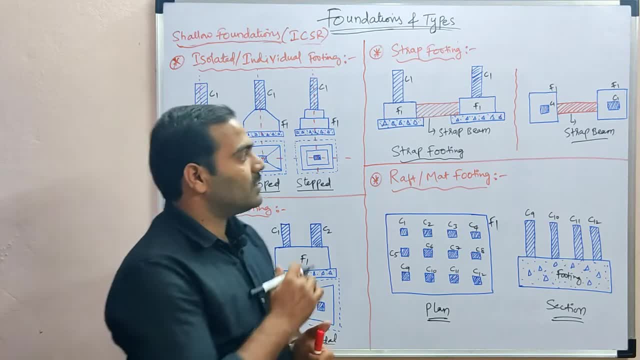 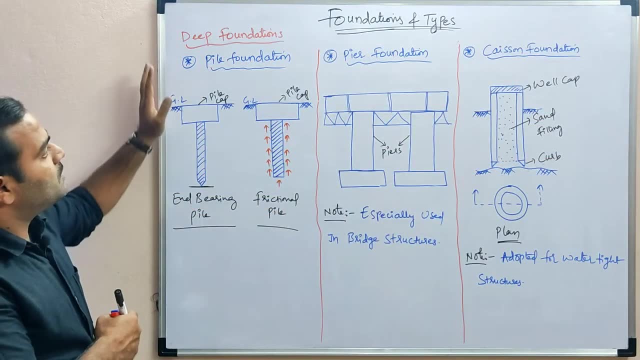 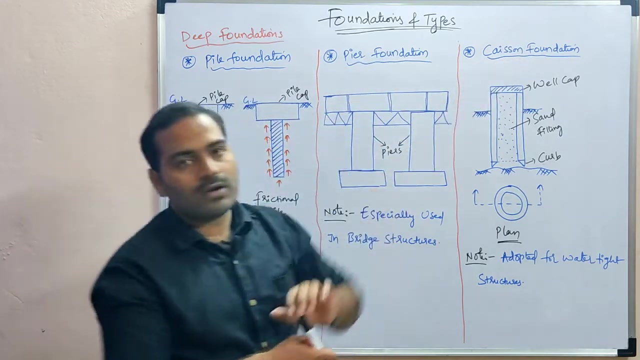 is called raft or mat footing. so these are all comes under shallow type of foundation. now we will see deep foundations also. so these are the different types of deep foundations. first one is pile foundation, second one is pier foundation and third one is caisson or well foundation. so if we take a first one, pile foundation, it is again divided into two. 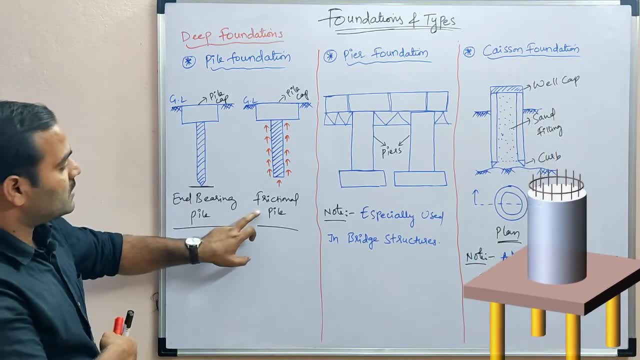 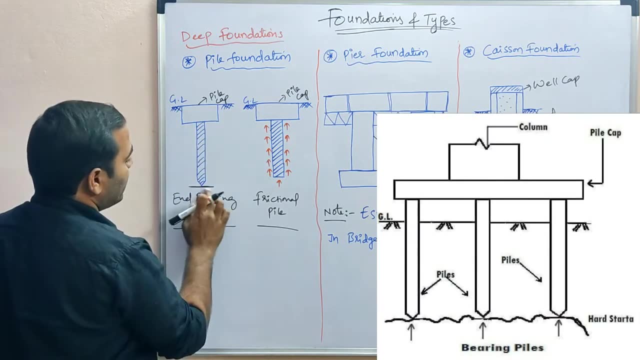 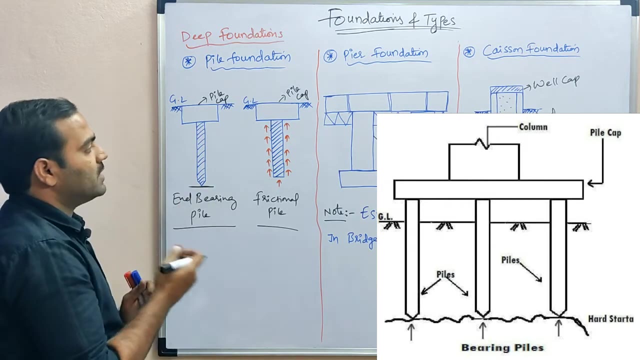 different types. first one is end bearing pile. second one is frictional pile. what is end bearing pile? so the complete load which is transferred through this pile will be bared by the bottom hard strata. so this load will be transferred to bottom hard strata, certain depths. so this type of pile is called end bearing pile and this type of pile is called 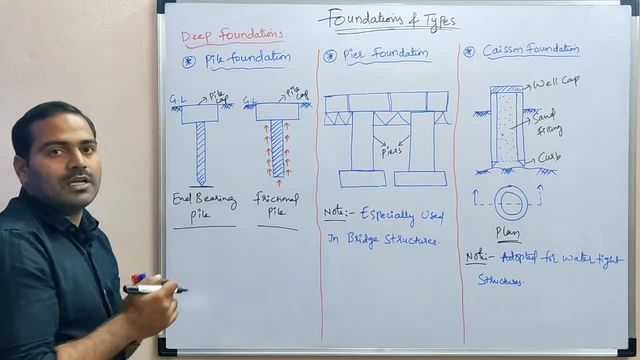 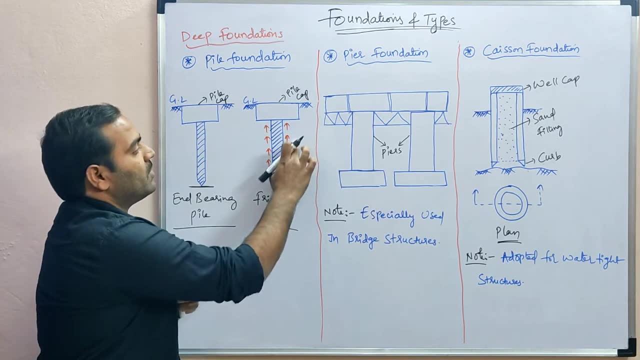 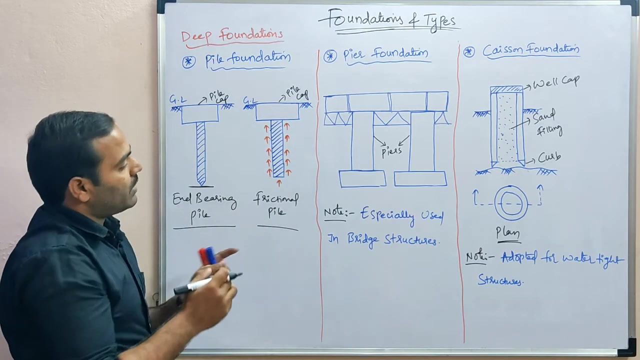 frictional pile because the friction is developed around the pile, so the soil, whichever is present around this pile, will be forcing upwards. that means upward forces acting from the soil so that this load will be transferred to the surrounding soil of this pile. so these are the two different. 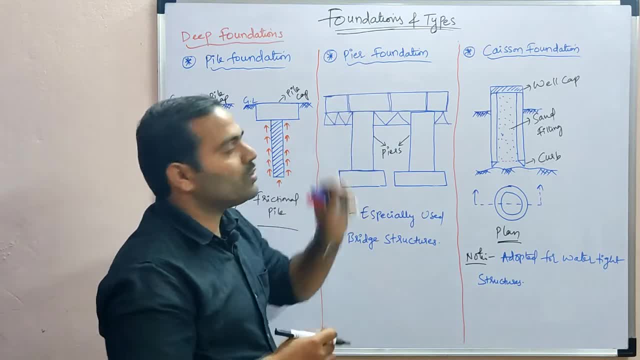 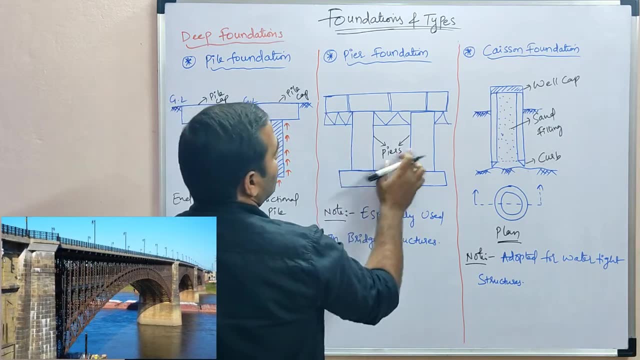 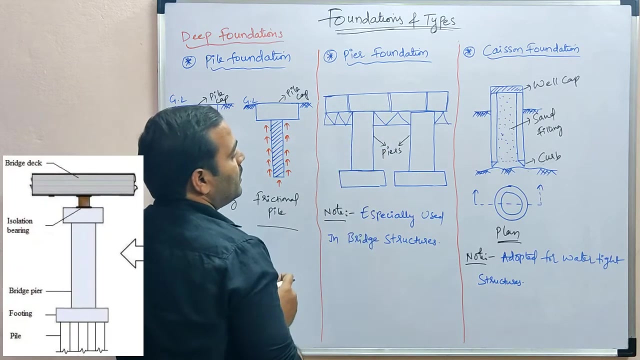 types of piles. and coming to pier foundation, mostly this type of foundation can be seen in bridges. so if we take a bridge, so these two are called piers and this is the bridge. so the load which is coming from the bridge will be transferred to this piers and it will be 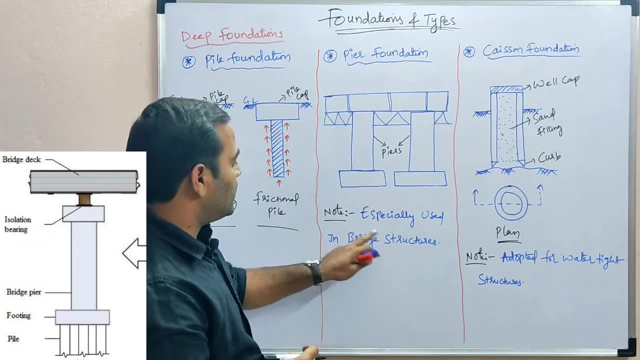 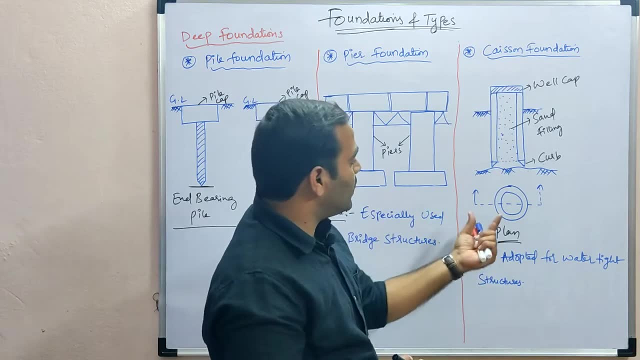 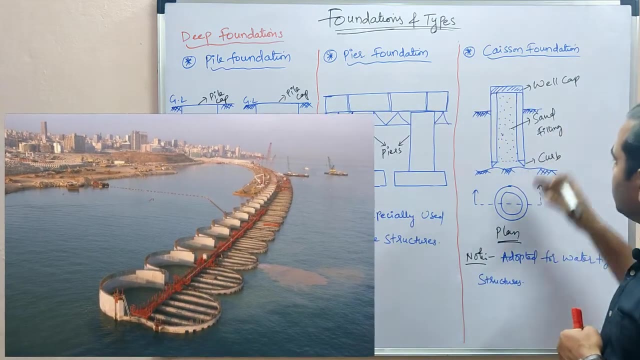 transferred to the subgrade. so especially it is used for bridge structures. so third type of foundation is caisson foundations or well foundations. this is completely used for water tight structures. that means where the water is more, water levels are more, then we are going to use this kind of caisson foundations. so if you see this, this will be.